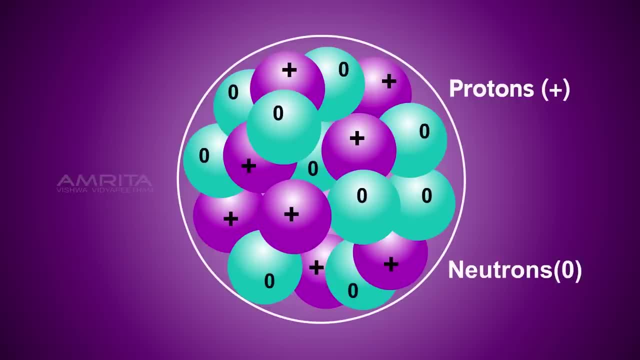 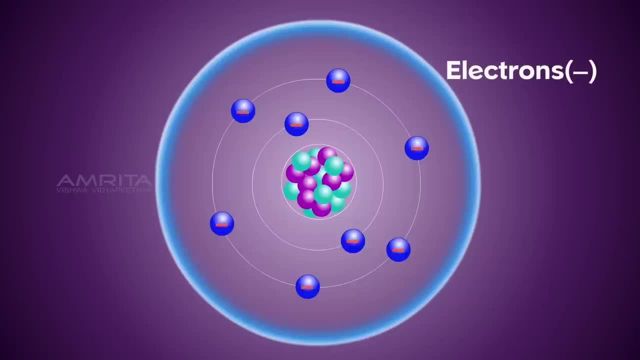 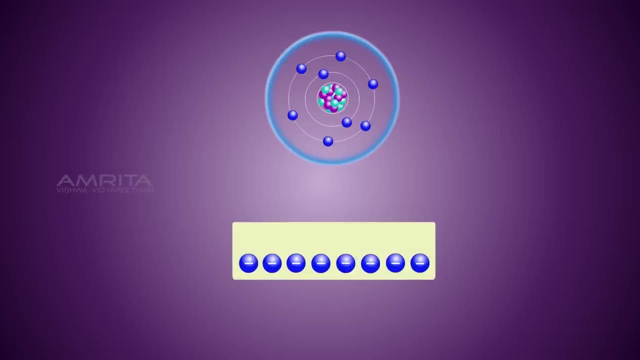 positively charged and neutrons have no charge. so the nucleus is positively charged. Protons and neutrons are collectively called nucleons. Electrons are negatively charged and are located around the nucleus. An atom has the same number of negatively charged electrons as it has. 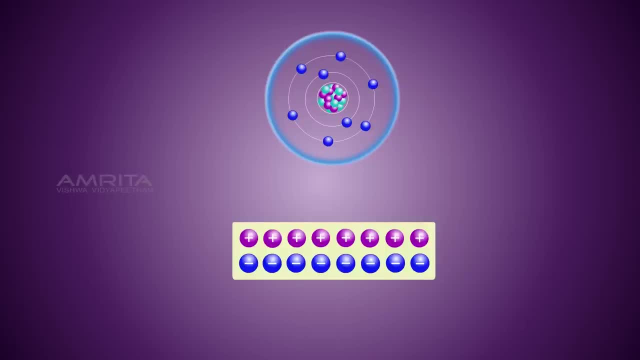 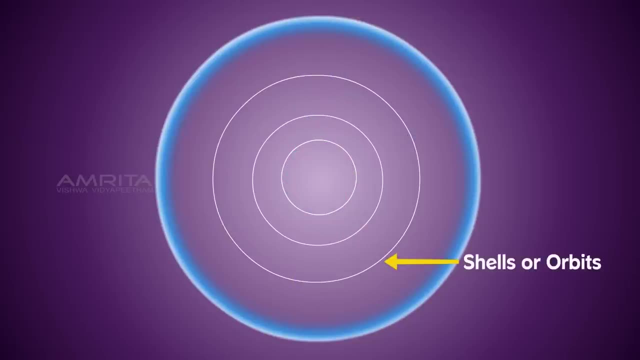 positively charged protons in the nucleus. Therefore, atoms are electrically neutral. Electrons are distributed in a definite path around the nucleus and are called shells or orbits. This concept was introduced by Niels Bohr. According to Bohr, different electrons 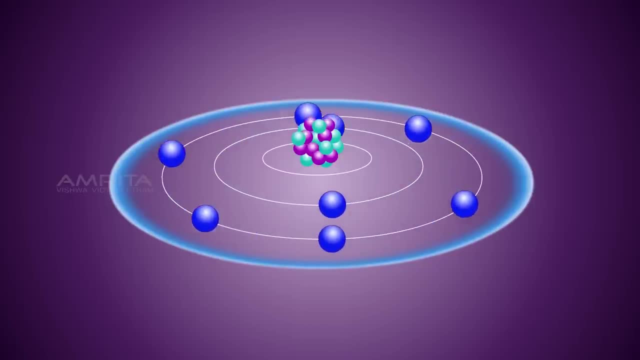 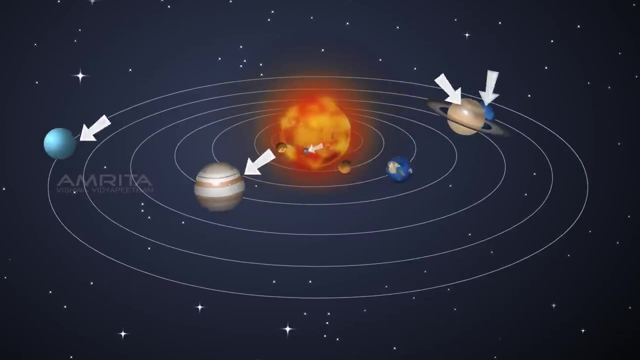 revolve around the nucleus in their own different orbits. The atom has been compared to the solar system. In an atom, the nucleus is the sun and the electrons are the planets, Just like planets in the solar system, each electron revolves around the nucleus in its own different. 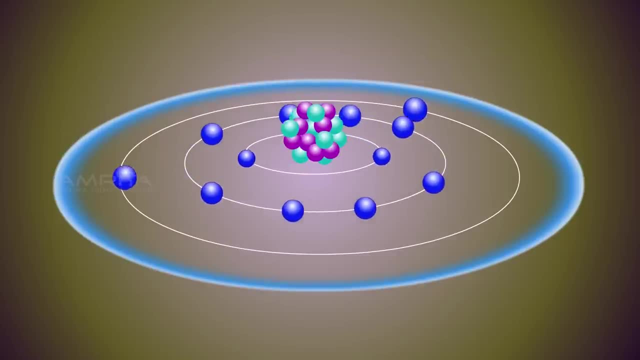 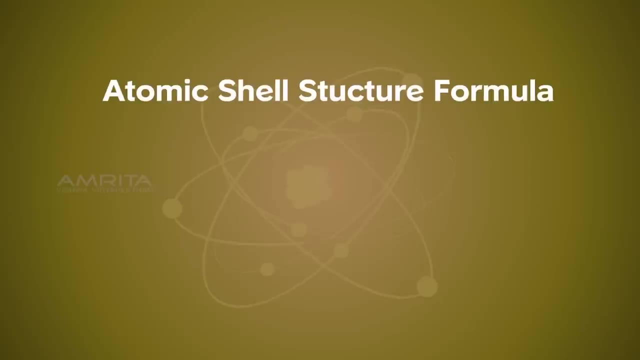 orbit. The orbits or shells are represented by the letters K, L, M, etc. The maximum number of electrons present in a shell is given by the formula 2N square, where N is the orbit number of energy cells. The first orbit or K shell can have 2, the second orbit, or L. 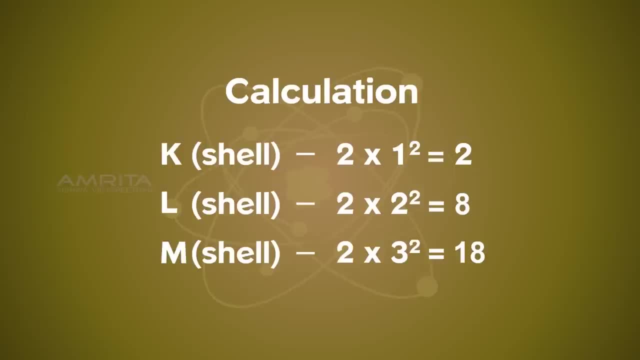 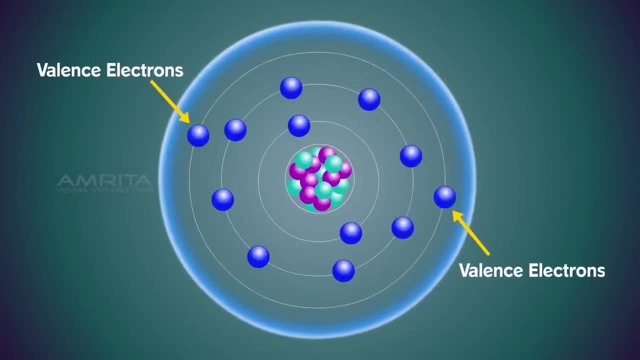 shell can have 8 and M shell can have 18 electrons, etc. The electrons present in the outermost shell of an atom are called valence electrons and the shell which valence electrons occupy is called the valence shell. A molecule is in. 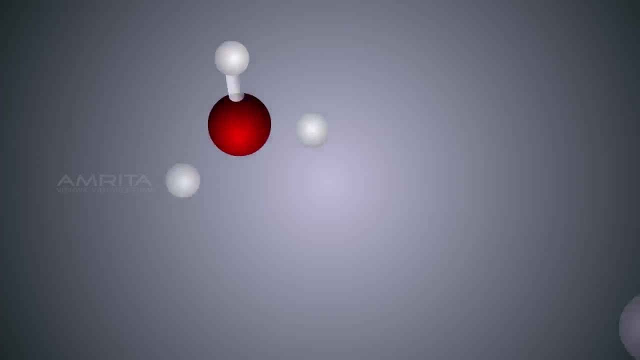 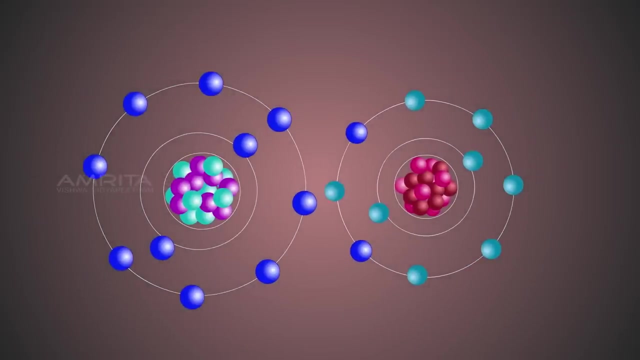 general, a group of two or more atoms that is chemically bonded together. Atoms combine chemically by external forces such as heat and light. This leads to the formation of molecules. During the formation of a molecule, atoms lose their valence, electrons or gain. 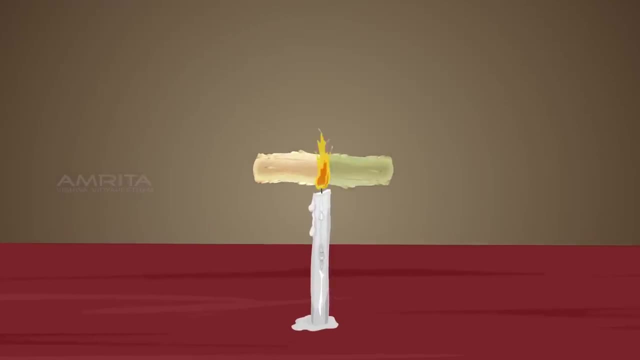 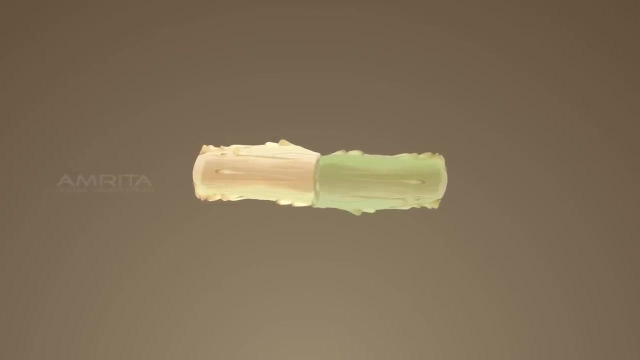 electrons from other atoms. For instance, if two pieces of wax are to be joined, they are heated. After heating, the two pieces are pressed together to form a single structure. Here, heat is the chemical factor which is responsible for joining the molecules of wax. 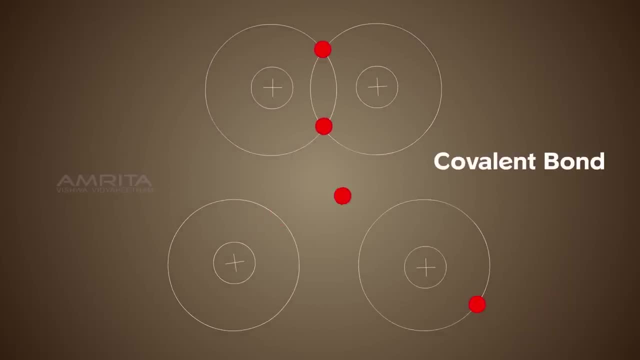 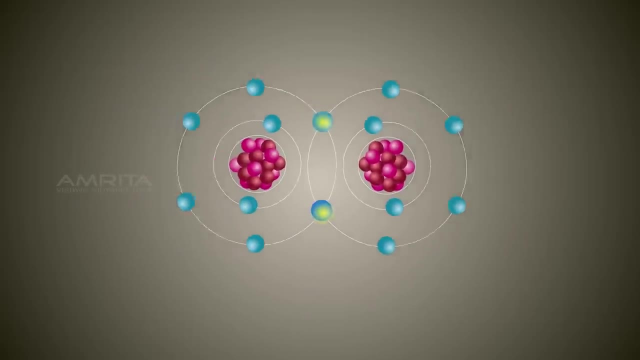 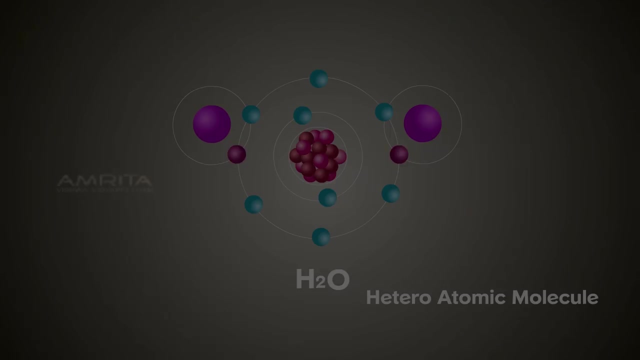 pieces. There are two main types of bonds: Covalent and Ionic. If a molecule is made up of atoms of the same element, it is called a homoatomic molecule. If the molecule is made up of atoms of different elements, it is called a heteroatomic molecule.